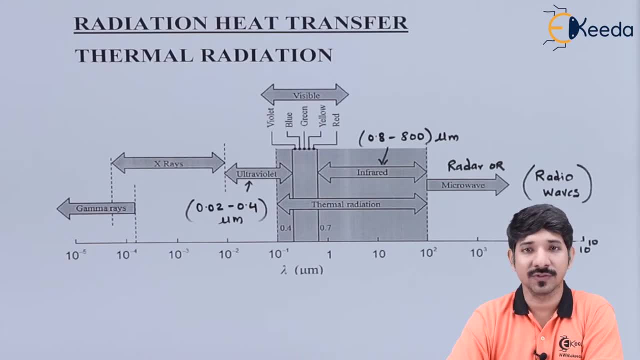 these kind of radiations or via these kind of electromagnetic waves. Now, this type of heat transfer is we code as a radiation type of heat transfer. Now, in our curriculum, out of all the electromagnetic waves that we need to consider as a radiation, there is only a small band of the wavelength which we are going to. 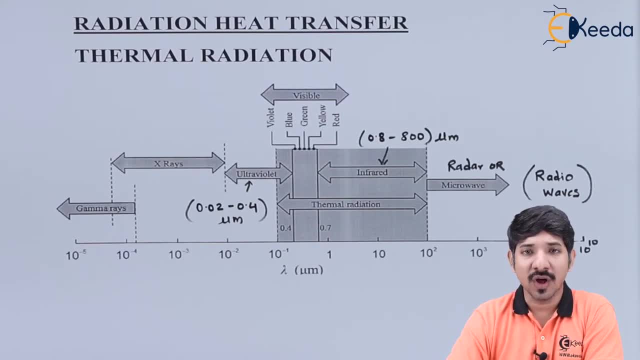 consider as a thermal radiation, because that small band of wavelength itself produces the heat. Now let us look at this diagram. In this diagram we have tried to write down the wavelength in terms of micrometer. Now, if the wavelength is very small, so it is in the range of, or even the lesser than, 10s to 5 micrometer, then that sort of 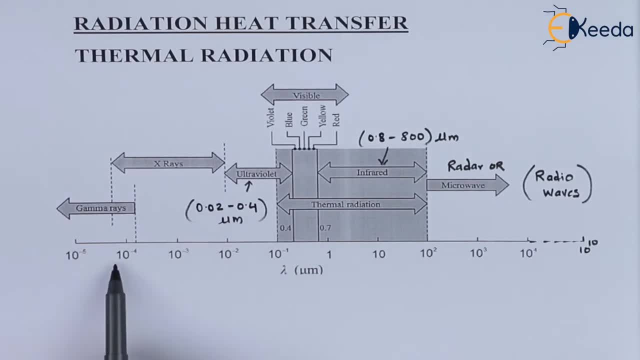 radiation we code as a gamma rays. Then between 10s to minus 4 and 10s to minus 2, we have the X-rays. Now the use of X-rays or gamma rays not. this is not there in our study. 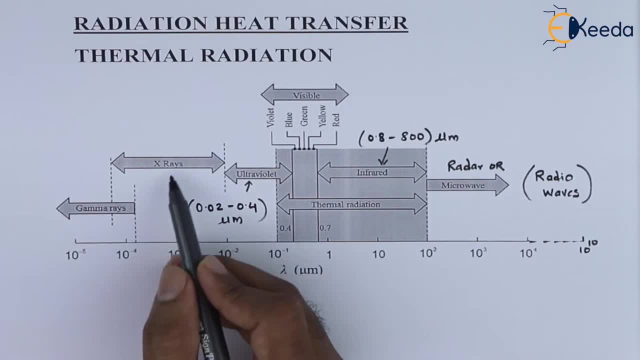 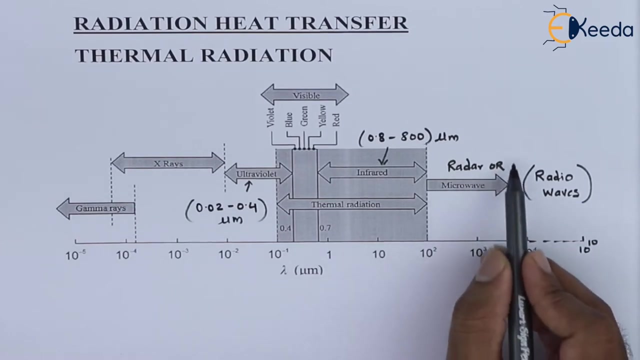 It is mostly used by the. some nuclear scientists are even further biomedical uses. So these are also categorized as the radiation, but are very low wavelength or very high frequency, then at the higher end. So any radiation that is more than to 2, we code them as a radar radiation or the microwave. So these radiations are also 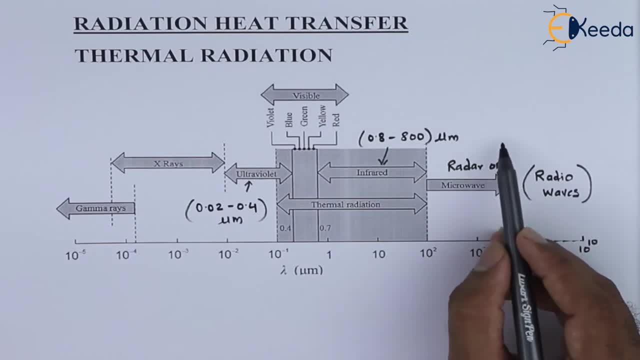 not there in the curriculum or they don't categorize themselves under the thermal radiation and any radiation more than 10 raise to 4 micrometer. we call them as a radio waves. Obviously they do not signifies in any the heat transfer. So for electronic engineer. 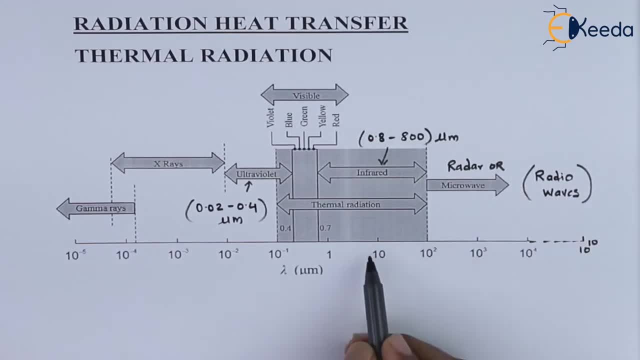 this wavelength will be of his interest, but we will be interested in this region. So that is between 10 raise to minus 1, so that is, let's say, 0.1 to 100. So between these two the radiation that we call are nothing but the thermal radiation. So any wavelength, 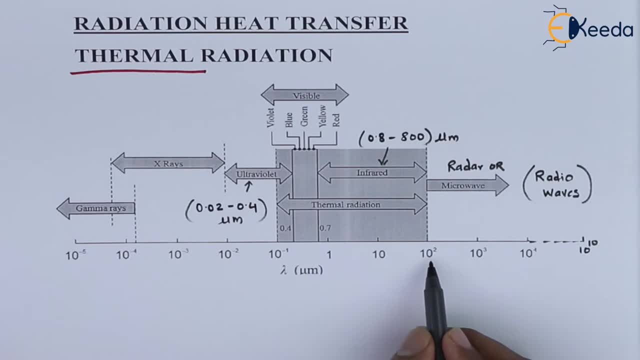 between 0.01 to 100 micrometer. those wavelengths come through the thermal radiation, So that comes under the category of the thermal radiation. Now, in that also we have got three categories. one is the UV rays, the ultraviolet rays. Now, these are the same rays by which we get